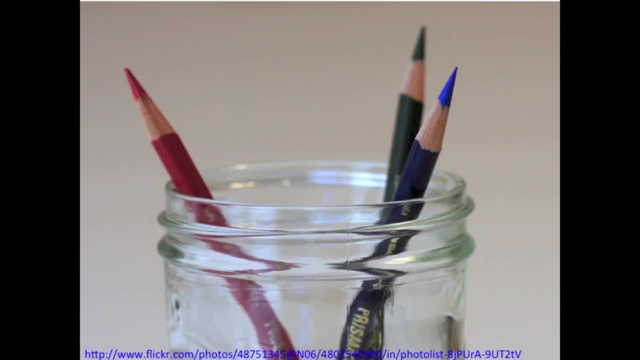 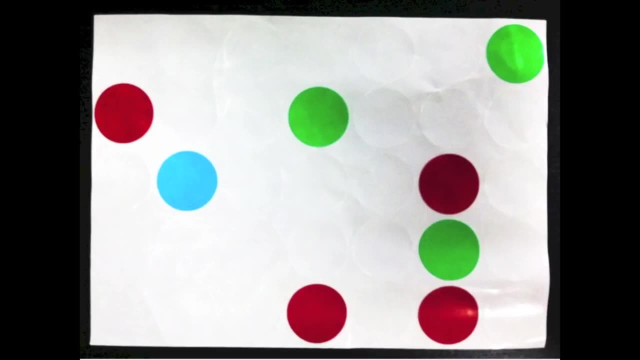 data helps us answer questions like how many blue pencils are in this jar Or how many black puppies are in this litter. Here is a picture of some of the stickers I have in my collection. Can you collect the data Count how many dots I have of each color? I have one blue sticker. 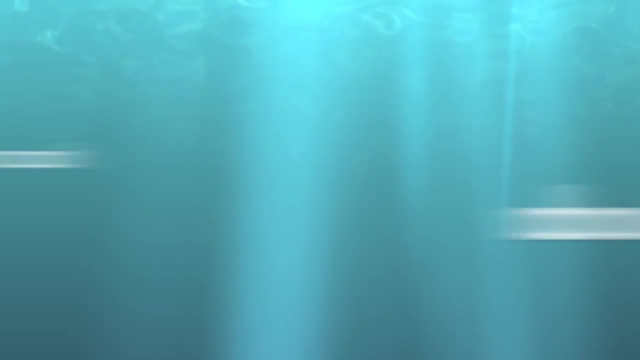 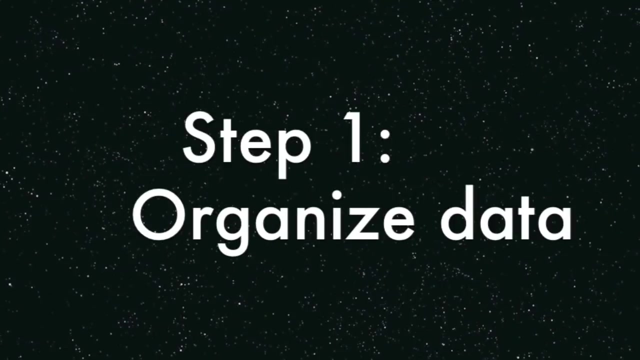 four red stickers and three green stickers. So what is so cool about data? Data helps you answer questions like how many blue pencils are in this jar Or how many black puppies are in this jar. What is so cool about data? Data helps you answer questions using numbers and facts. Step one: 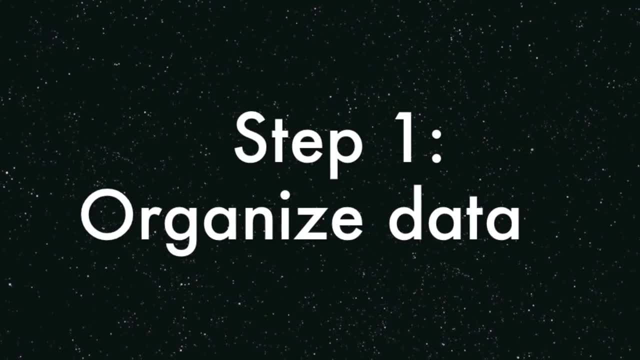 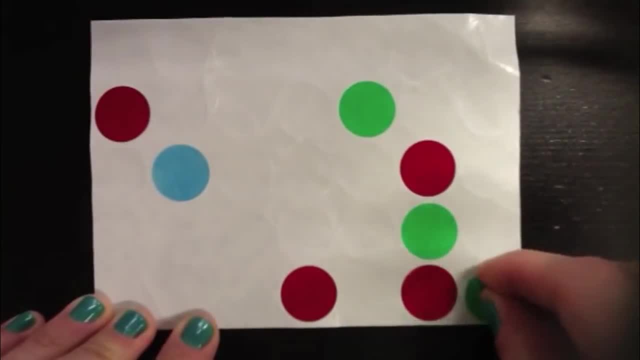 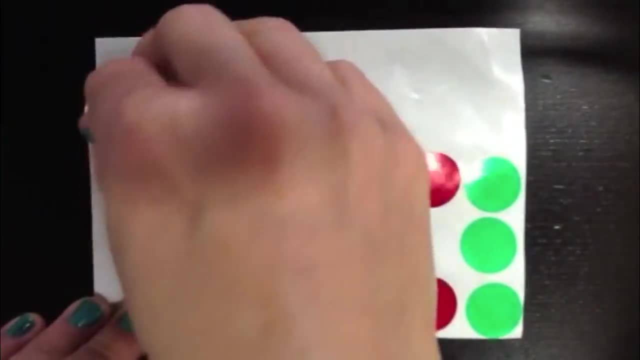 is organizing the data. Let's organize the data from my sticker collection. Let's start with the green stickers. I'll put them all in one line so that they're easy to count. Now let's organize our red stickers. We can line them right up next to our green stickers. Last, 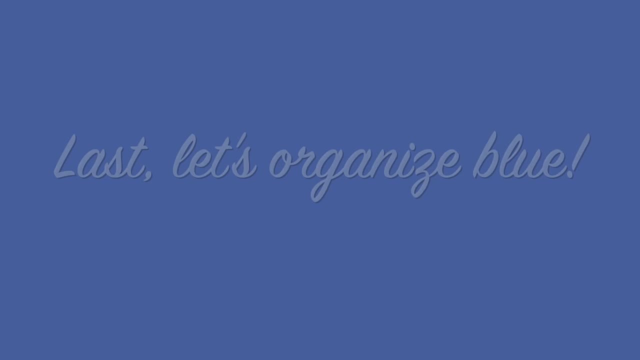 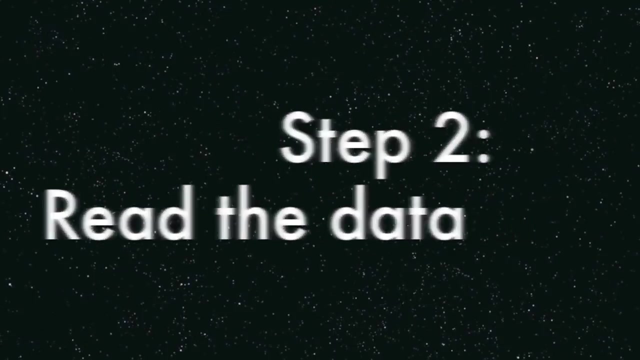 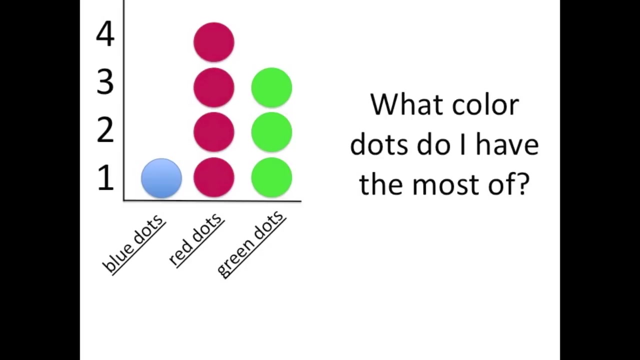 let's organize our blue sticker. Let's put it in line with the rest of the dots. After we organize our data and put it in a chart, we have to read it When our data is in a chart. it makes it easy to answer questions like this: What color dots do I? 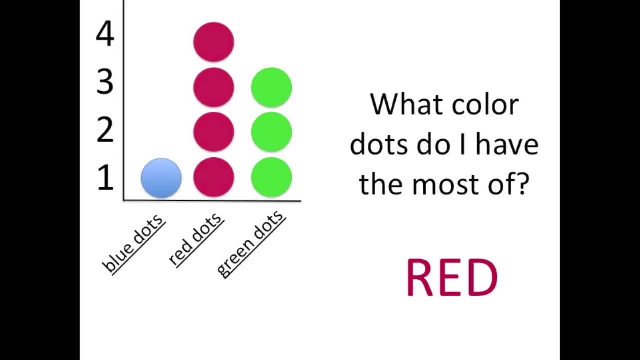 have the most of? I have the most red dots From my chart. can you figure out how many green dots I have? I have three green stickers From my chart. can you tell what color sticker I have the least of Blue? Looking at all of our data in a chart helps us answer all of. 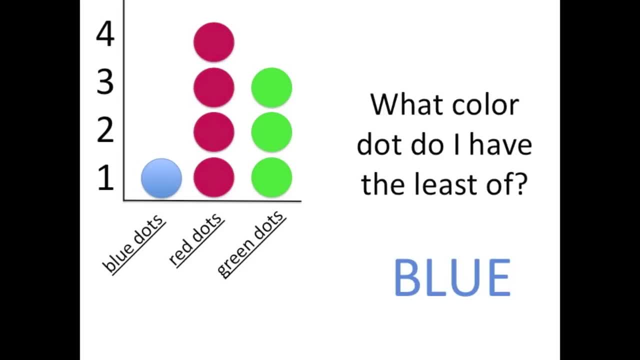 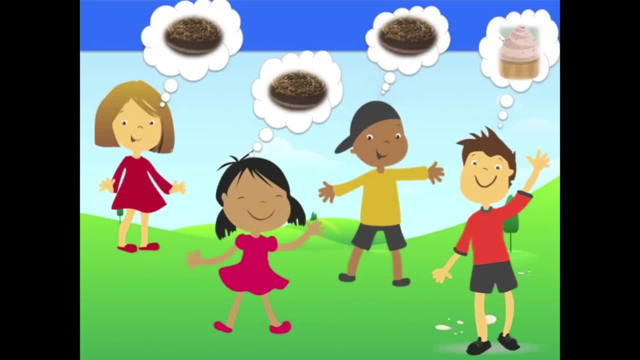 these questions about the numbers we're dealing with. Now let's organize this data. I polled all of my friends to see what kind of dessert they liked best. I like cookies the the best. Athena and Xavier also really like cookies, and Elliot's favorite dessert is cupcakes. So first let's count the data. 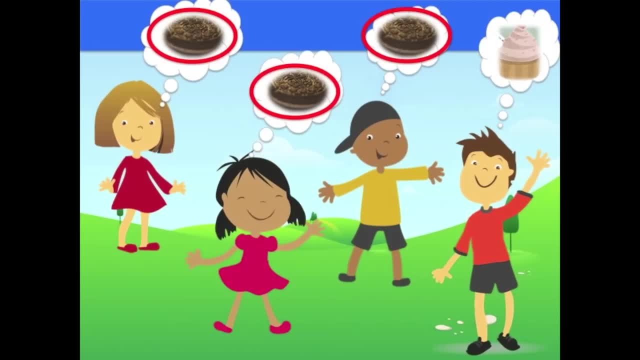 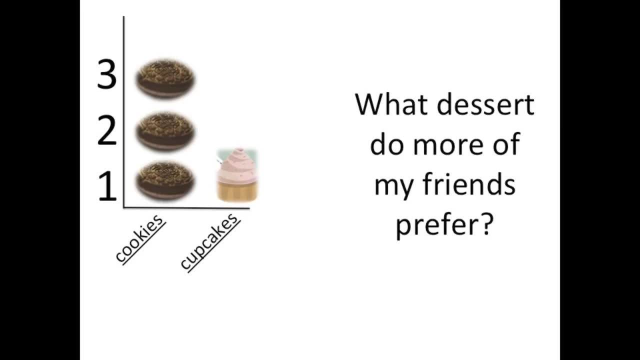 1..2..3 people like cookies the most. one person likes cupcakes the most. I organized my data so that I could tell that three people like cookies the most and one person likes cupcakes the most. now someone can look at this chart to answer the question: what dessert do more?